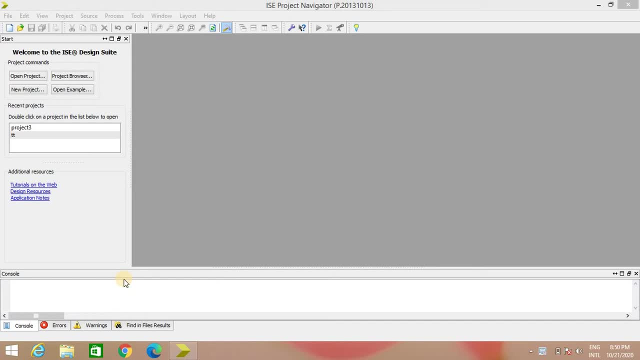 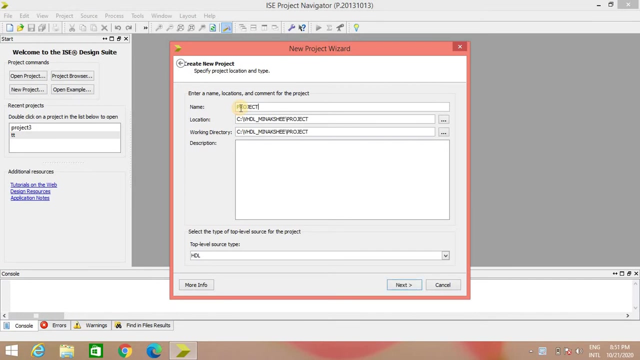 Welcome all. In this video we will discuss simulation flow for Xilinx IRC Design Suite 14.7.. For that I will elaborate simple and basic VHDL code for ANDGATE. Let's start. Click on File New Project. Give Project Name. I have given the name Project Basic. We can. 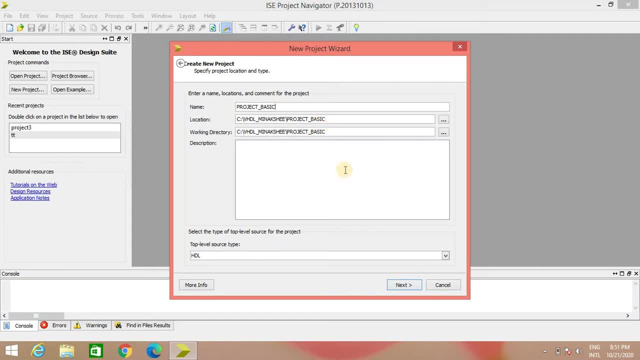 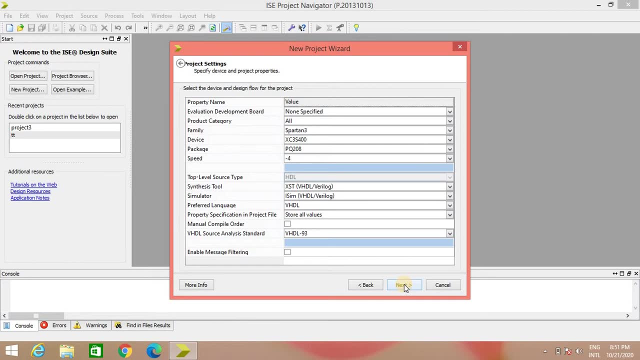 decide the location where I want to store this project and then Next In this window we can select the properties for the device that you want that we want to use for the project. So Product Category is All. Family we are using is Spartan 3.. Device is XC3S400.. 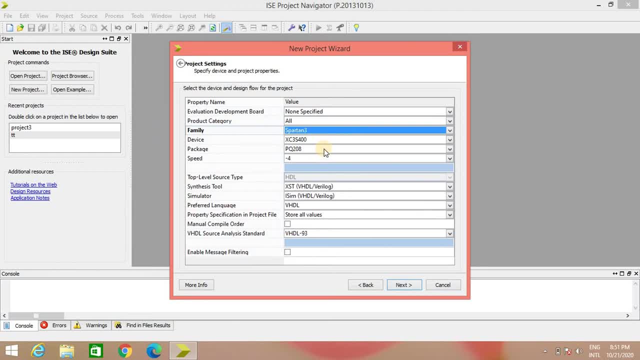 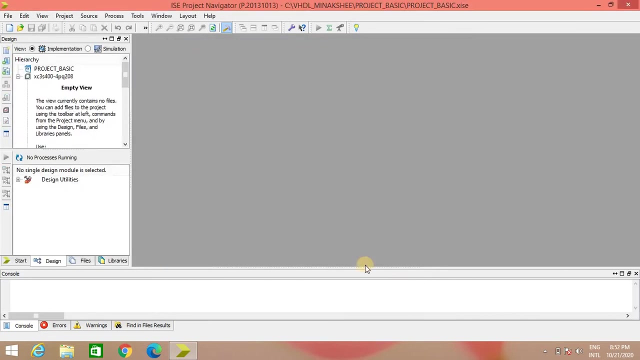 Package is TQ208.. And here we can select the hardware language. We have two options: We can go for VHDL or we can go for Verilog. So here we are selecting VHDL And here click on Next, Then Finish. Here you can see the same device that you have selected. 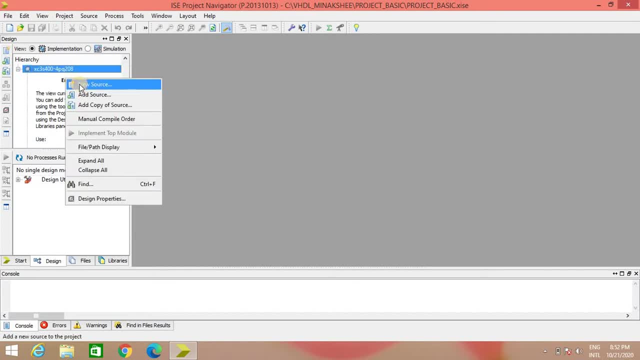 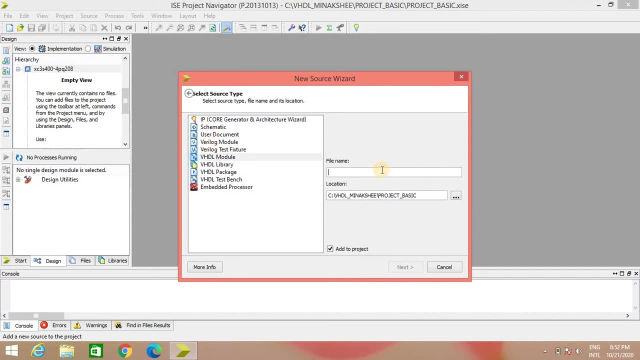 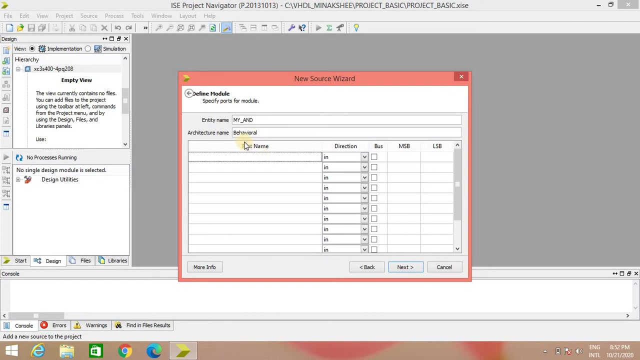 for your project. Right click on it, New Source. Then select VHDL Module, Give the file name. This file name is same as your entity name, So I am giving the name as myANDGATE And Next Now in this window we can give detail of entity name. We can see the architecture. 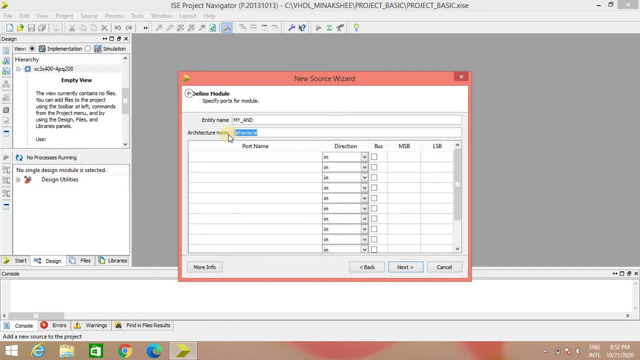 name as well. Here, if we want, we can change the name. I am changing it to the data flow. Here we can write the name of the ports that we are using. We can decide whether it is input or output port, And then here we can decide the size of that port as well. So I am giving the name as 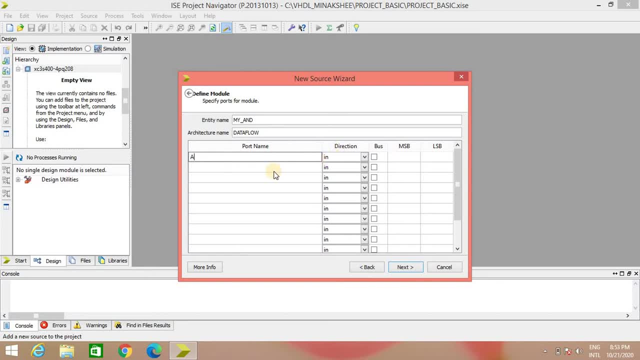 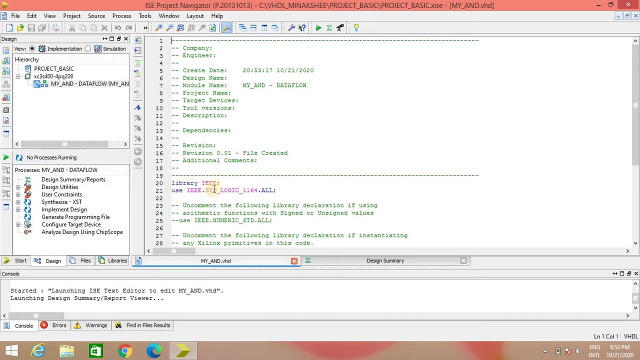 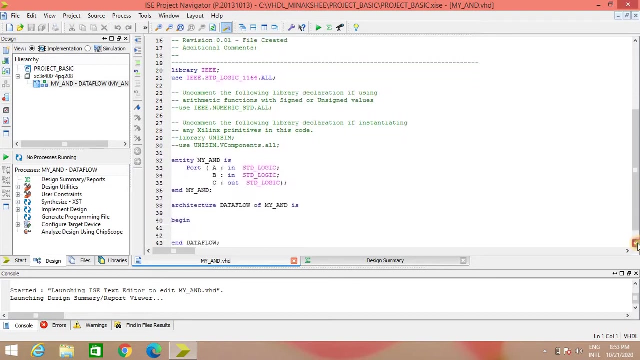 A, That is input, Then B, Again input, And C As output, Next Finish. So a new window will open in front of you Where you can see the library section. Then we can see the entity section as well. So 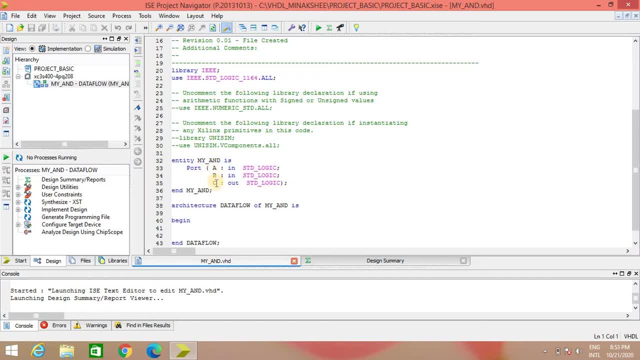 here, entity is myAND. A, B, C are the ports And their direction is in, in and out. Then we can see the architecture. The name of the architecture that we have given is data flow of entity name myAND. After begin, I can write my code. 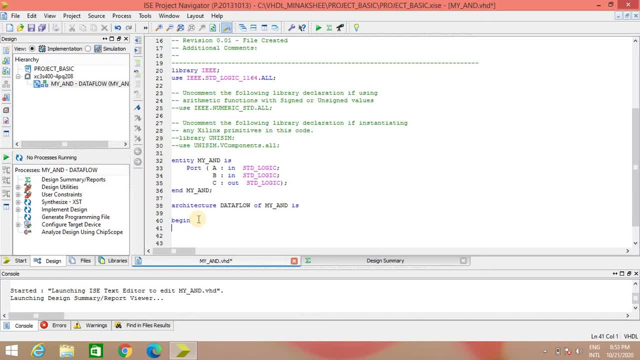 It is a simple code for the AND gates. So I am writing C assign with A AND B. So here, simply, we are taking two inputs, We are ANDing that and the output result we are giving for the C. Save your code with control S. And now your next step will be checking the syntax. 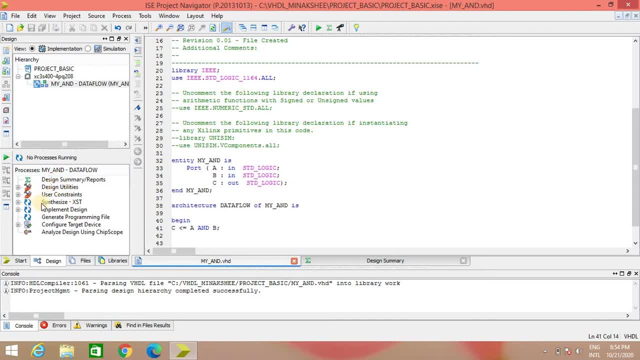 For that. Save your code with control S. And now your next step will be checking the syntax For that. Save your code with control S. And now your next step will be checking the syntax For that. Select, synthesize, XST, Explore it. Check for the check syntax option: Double click it. 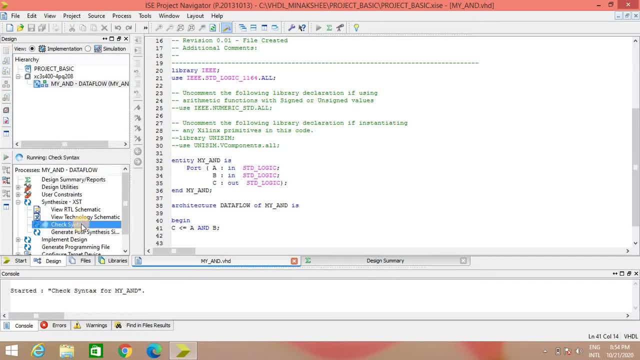 So it is showing green tick. It means there is no syntax error in our code. So it is showing process check: syntax completed successfully. Now the next step will be: We have to see what hardware is generated for our code that we can see with view rtl schematic option. 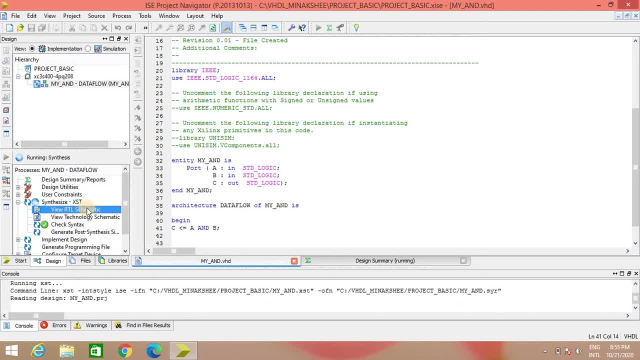 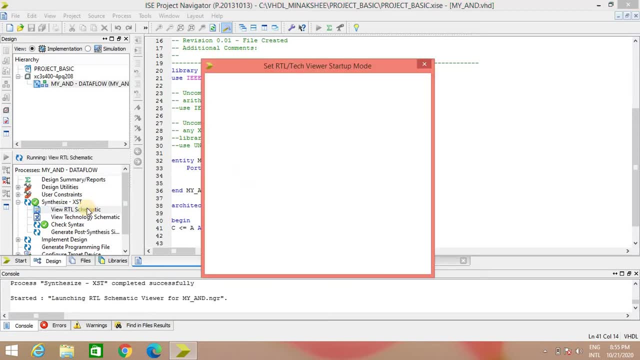 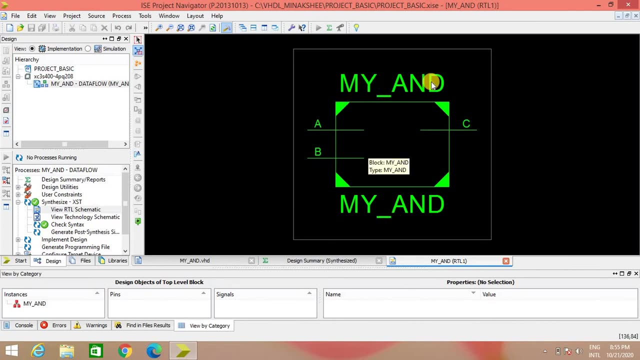 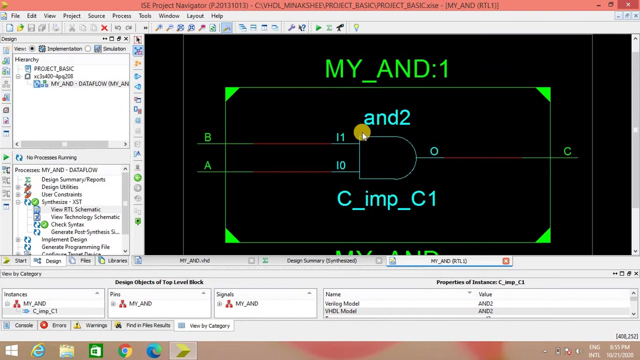 double click on that. click ok. now here you can see the entity diagram. you can see the entity name, my, and a and b are the input, whereas c is output. click inside and you can see a and gate. that is generated as a result of the code you have written. so 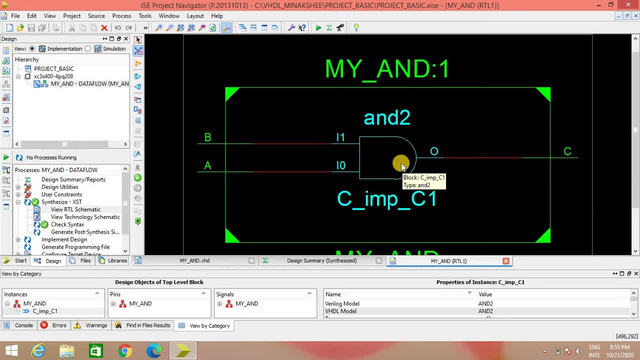 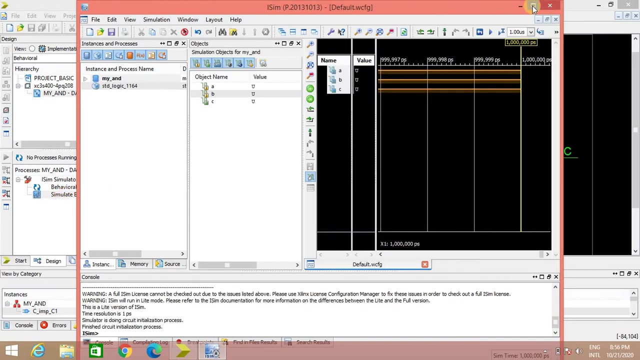 it is successfully generated. now we have to simulate the hardware that is generated. for that we will go for option simulation. ok, select the entity, then select simulate behavioral model, double click ok. so in this window we can see that we have selected the code which is generated for our code. 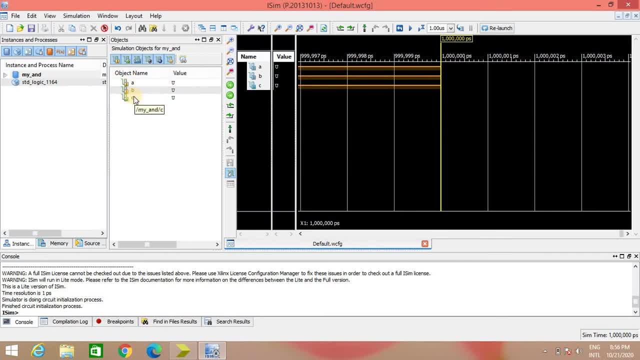 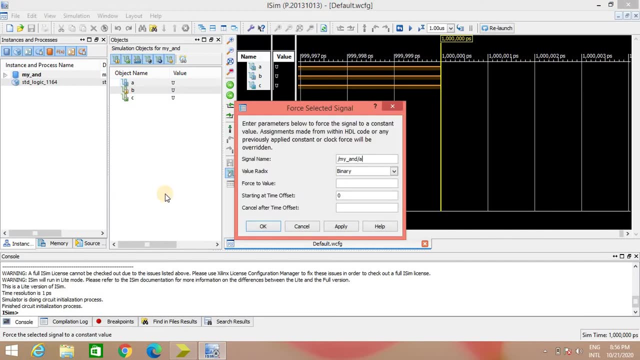 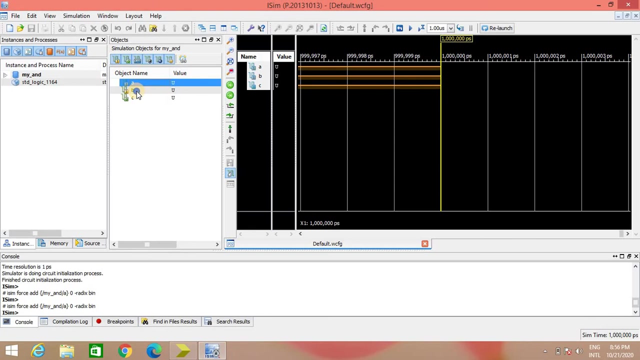 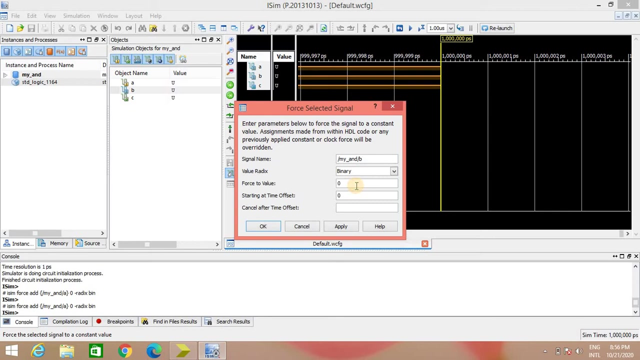 We can see all the object names: a, b and c. Initially they are undefined because we have not given any value to it. So let us give some value. Click on a right click force constant. give value to a as 0, apply ok. Give value to b. force constant: again 0,. 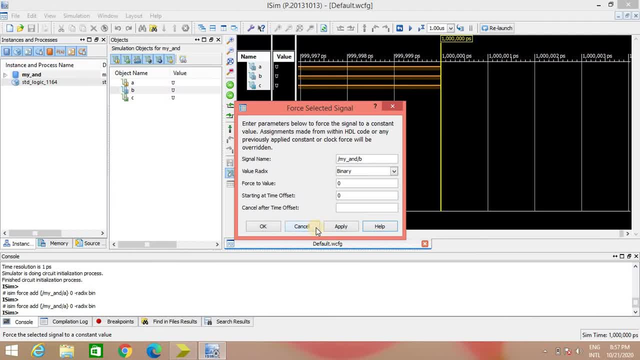 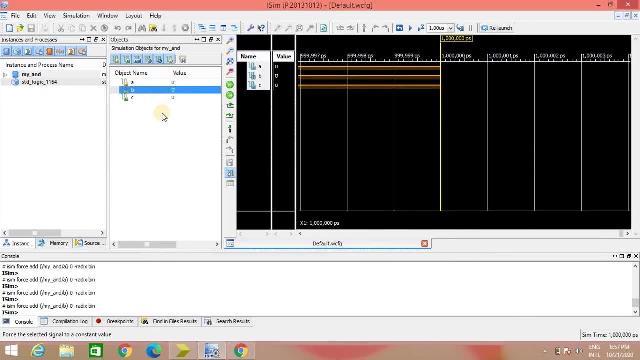 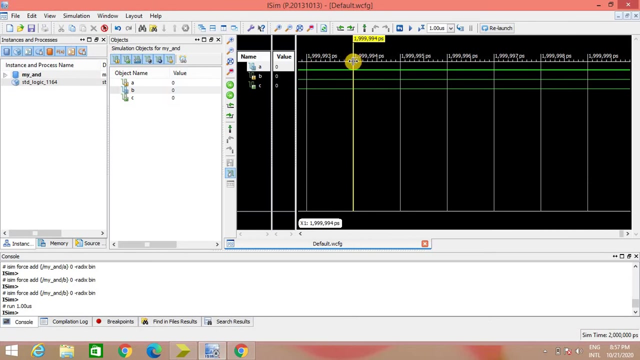 apply, apply, Ok, And then we will simulate it and for that we will click on the option run for the specified time. Click on that and here you can see the result. So what the result is showing When a is 0, this is called as marker. So marker is showing the position where you are reading. 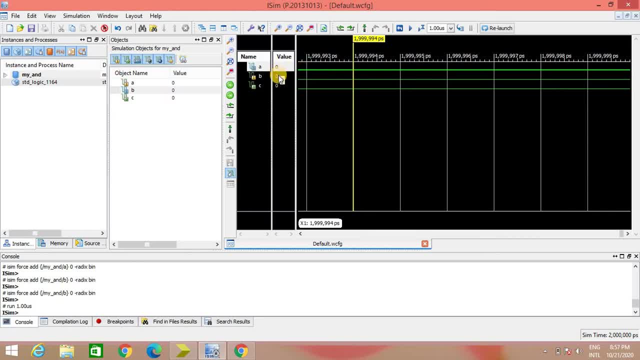 your values. So here you can see a is 0, b is 0, c is 0. So here you can see a is 0, b is 0, c is 0. So here you can see a is 0, c is 0, c is 0. So here you can see a is 0,. 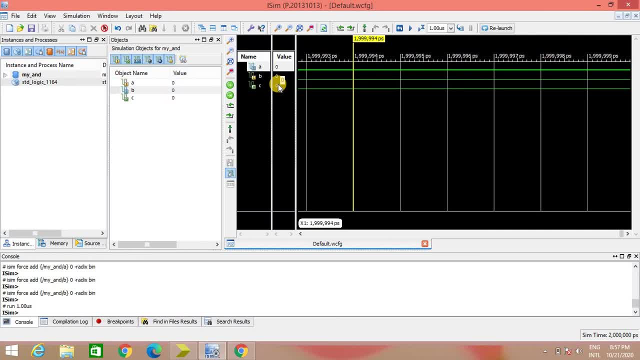 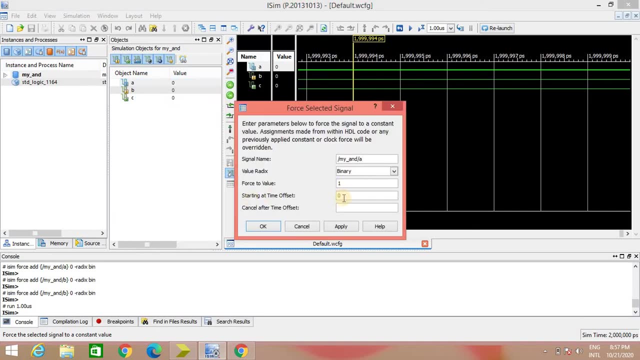 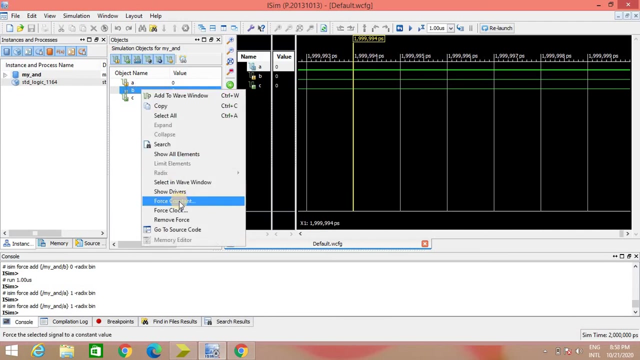 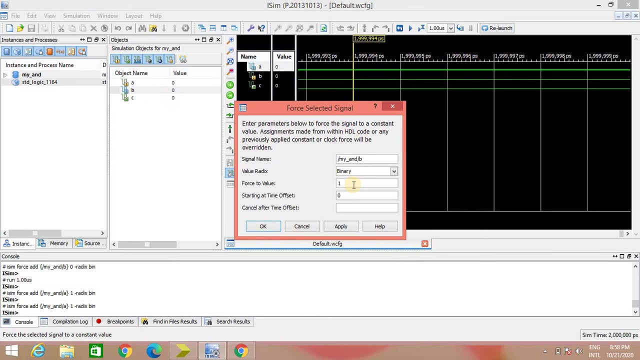 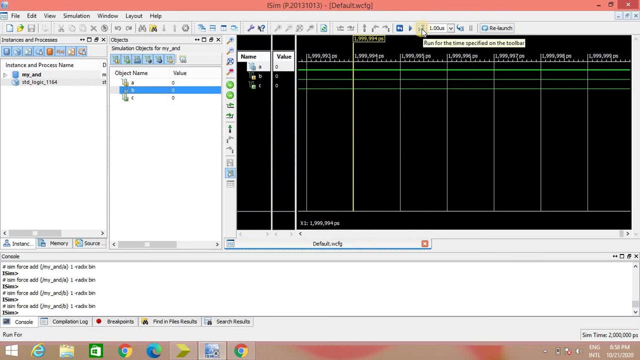 b is 0 and that time I am getting output as 0.. Now let us give some new combination for input Again. right click force constant value for a: I am giving as 1, apply ok. Right click force constant value for a: I am giving as 1, apply ok and run for the specific time.